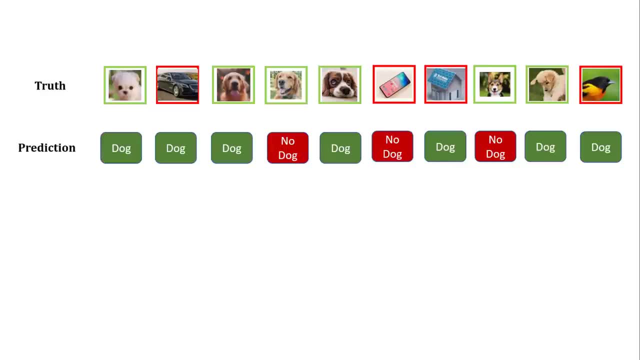 prediction. this is a prediction, hence it will not be true. it will be making some mistakes, okay. so now let's first. I have grayed out no dog predictions, okay. so we just think of predictions as your base and let's only talk about positive predictions, which is 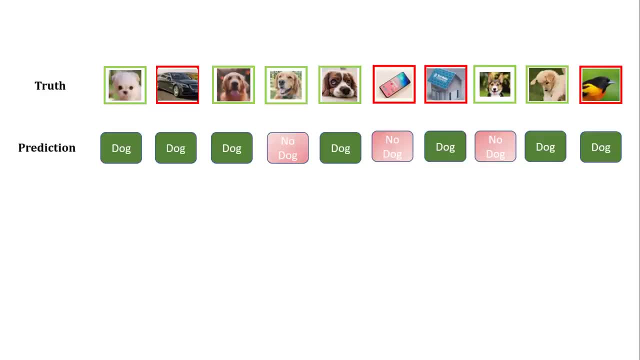 dog. okay, that's why I'm graying out this: no dog predictions, okay, so forget those no dog predictions for now. and you have now our total. seven are dog predictions. out of those seven, how many of them are correct? well, one: this is not correct. this is correct, okay. 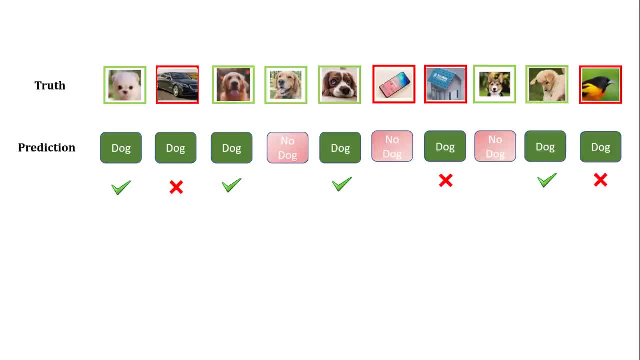 so you have classified, you have basically marked your prediction as correct or not correct. okay, for your positive class, which is dog, whichever predictions are correct here are called true, positive. so here the positive thing, which is the second word, means your class, our positive class, which is in: 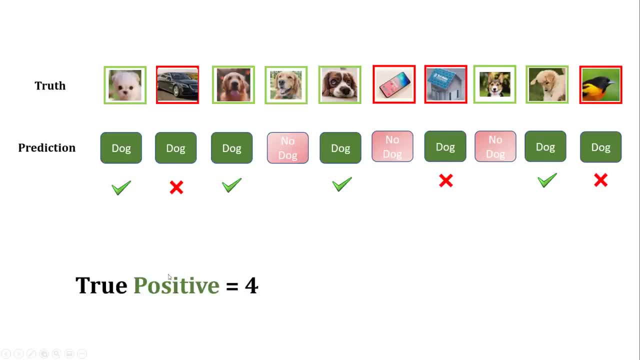 green is dog. so out of those positive prediction, how many of them are true, real? so when you try to identify them as true, you compare it with reality. so when we compare all this with reality, we found only four predictions were true for dog and three were wrong. so those are called false positives. so this again. the second: 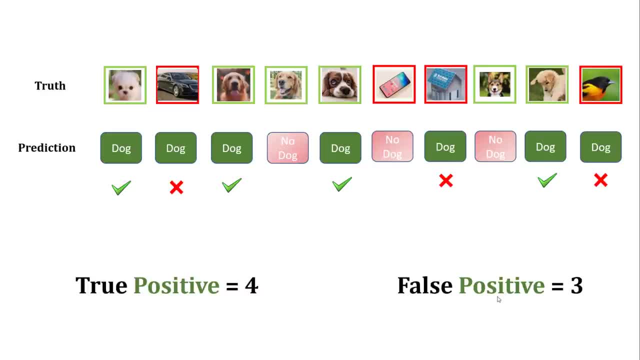 word positive indicates what the outcome of your prediction. okay, the outcome of the prediction was for these three samples which are red mark was positive, but they are false. so the first word indicates the reality. in reality they are false. okay, now think about no dog predictions. okay, so forget. 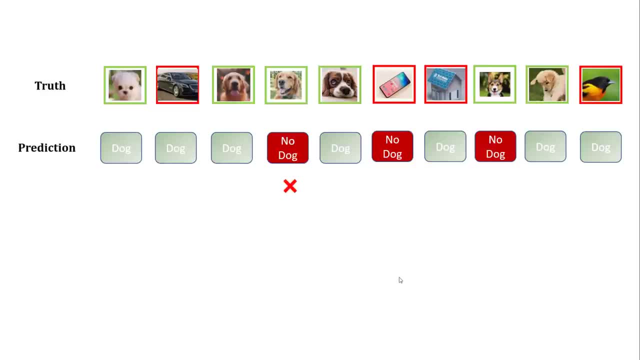 all those greens. that's why I have grayed it out. so here again I will go and compare all these three predictions with the reality. so two of these predictions are right, two of these are wrong and one is right. so true negative here is called one the. 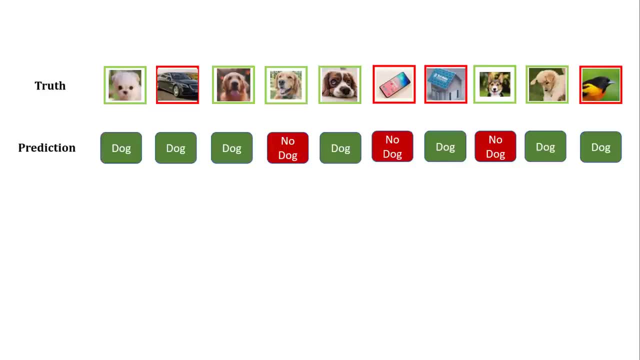 prediction. this is a prediction, hence it will not be true. it will be making some mistakes, okay. so now let's first. I have grayed out no dog predictions, okay. so we just think of predictions as your base and let's only talk about positive predictions, which is 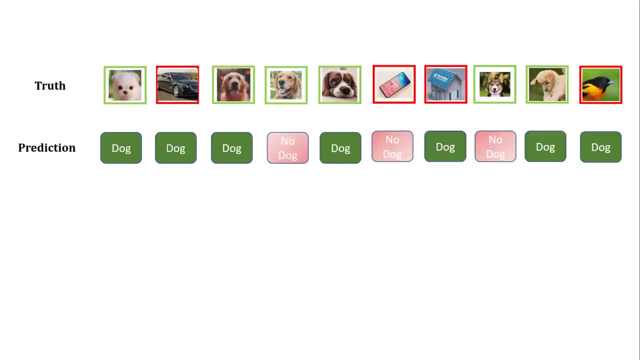 dog. okay, that's why I'm graying out this: no dog predictions. okay, so forget those no dog predictions for now. and you have now our total seven, our dog predictions. out of those seven, how many of them are correct? well, one: this is not correct. this is correct, okay. 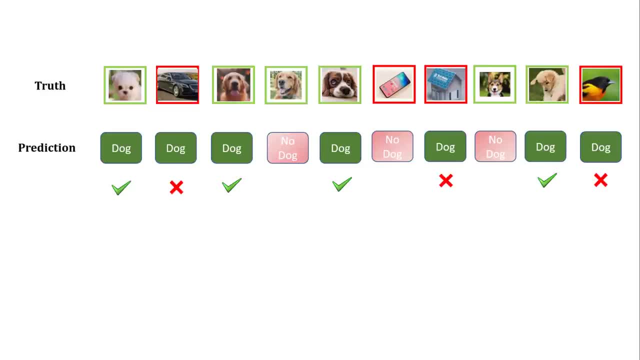 so you have classified, you have basically marked your prediction as correct or not correct. okay, for your positive class, which is dog, whichever predictions are correct here are called true, positive. so here the positive thing, which is the second word, means your class, our positive class, which is in: 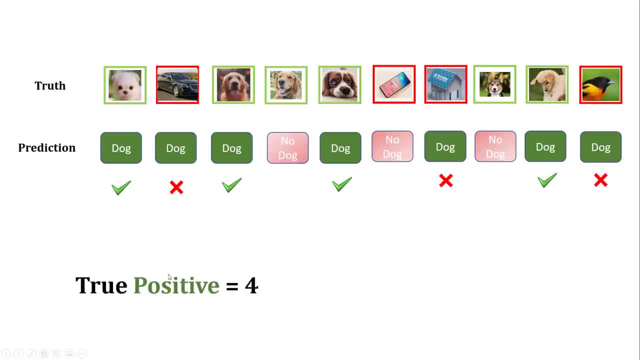 grain is dog. so out of those positive predictions, how many of them are true really? so when you try to identify them as true, you compare it with reality. so when we compare all this with reality, we found only four predictions were true for dog and three were wrong. so those are called false positives. so this again. the second. 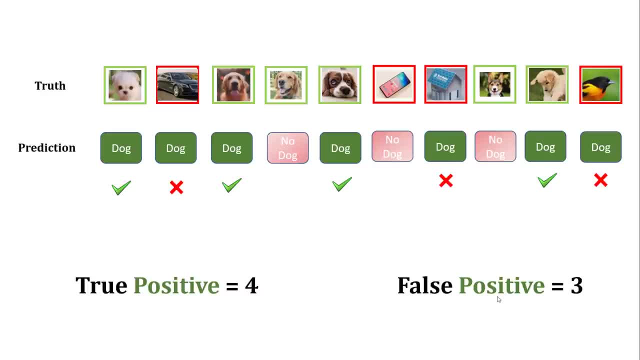 word positive indicates what's the outcome of your prediction. okay, the outcome of the prediction was for these three samples which are red mark was positive, but they are false. so the first word indicates the reality. in reality. they are false. okay, now think about no dog predictions. okay, so forget all those. 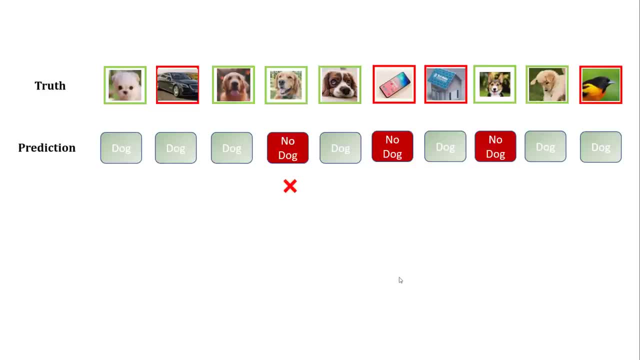 greens. that's why I have grayed it out. so here again I will go and compare all these three predictions with the reality. so two of these predictions are right, two of these are wrong and one is right. so, true, negative here is called one the negative. the second word means your class, which is no dog, which is, which is 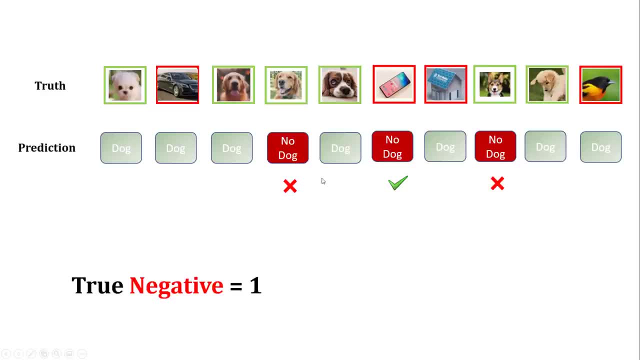 negative. the second word means your class, which is no dog, which is, which is negative class, right in our case. and out of these three predictions, only one was true. that's why it's called true negative is one and false negative is true. basically, out of our three negative predictions, two are false. 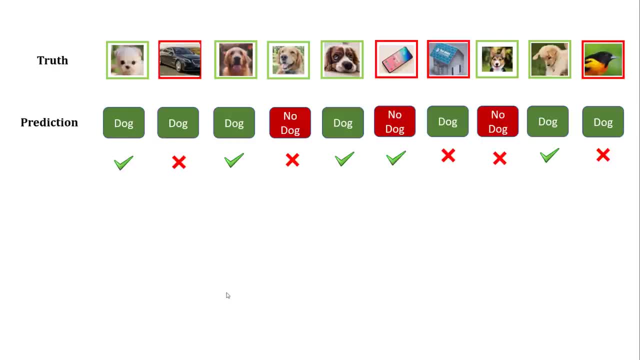 so now I have marked all my predictions here. so basically this shows out of all my predictions which predictions are correct and which are wrong. okay, so we got total five right and that is called accuracy. how many of your predictions you got right doesn't matter positive or negative predictions. how many of your 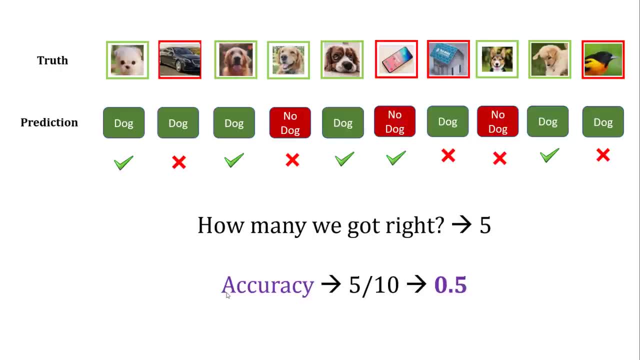 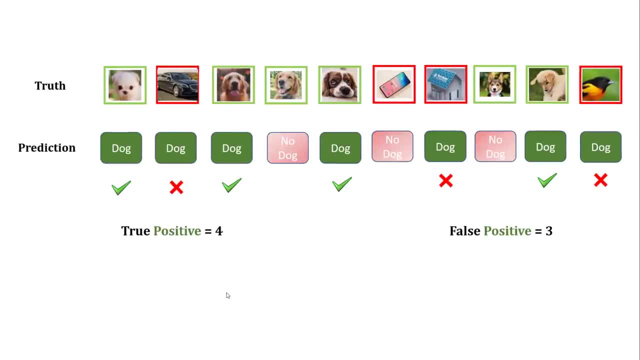 predictions. you got it right, so we got 5 out of 10 right hand and hence accuracy is 0.5. okay, now in this diagram again we are going back to only positive class. so forget the no dog prediction, just take those out of your visualization. here we saw true, positive. 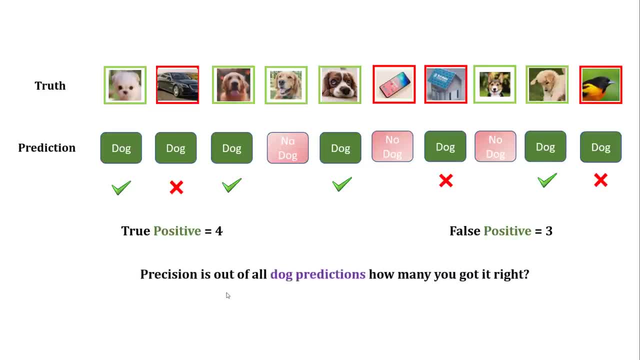 was 4 and false positive or 3, so precision is out. of all dog predictions, how many you got it right? so it is 4 by 7, so you have total 7 dog predictions right. 7 things you predicted it to be dog. out of that, only 4 are dog. so that's. 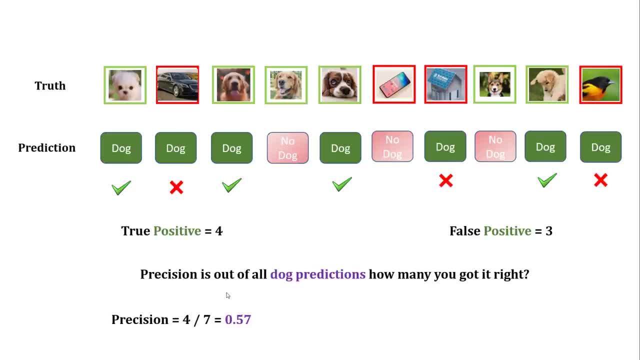 why precision is 4 by 7, point 57. so this is the formula for precision: true positive divided by true positive, false plus false positive. okay, now let's talk about recall, so that when you are thinking about recall, you always think about truth as your baseline. so what is? 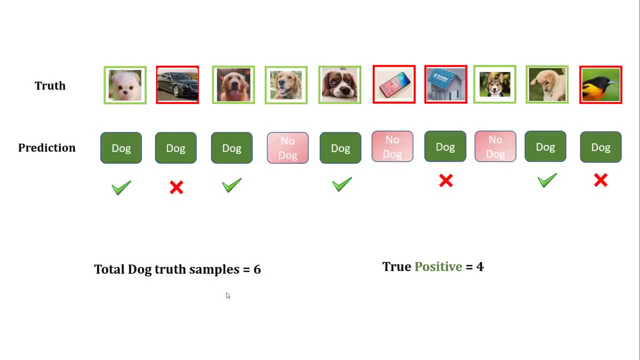 my truth, my, in my truth, total six samples are dog samples. okay, but when I predicted only I got four as correct prediction. so what is my truth? in my truth, total six samples are dog samples, predictions for dog. so recall, is, out of all your dog truth samples, how many you? 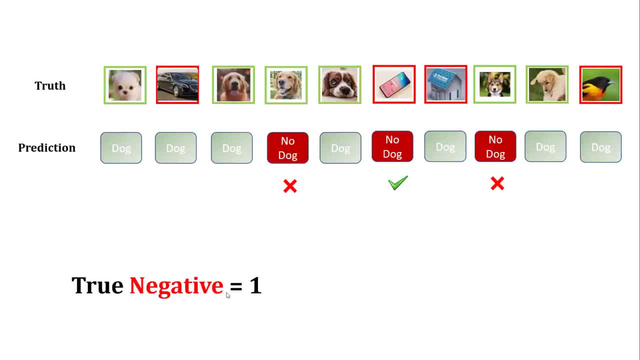 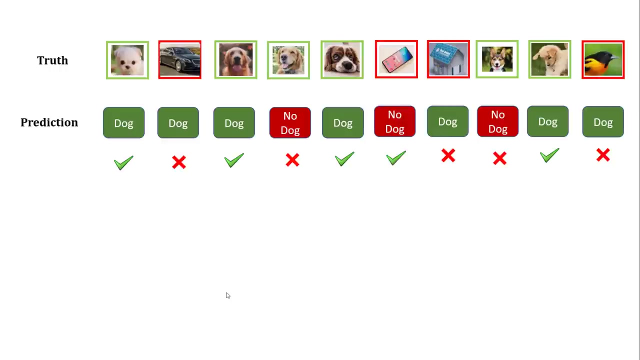 negative class, right in our case. and out of these three predictions, only one was true. that's why it's called true negative is one and false negative is two. basically, out of our three negative predictions, two are false. so now I have marked all my predictions here. so basically this shows out of all my 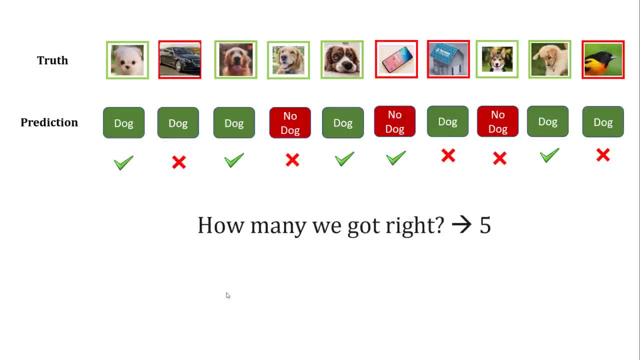 predictions: which predictions are correct and which are wrong. okay, so we got total five right, and that is called accuracy. how many of your predictions you got right doesn't matter positive or negative. right, and that is called accuracy. how many of your predictions you got right doesn't matter positive or negative. 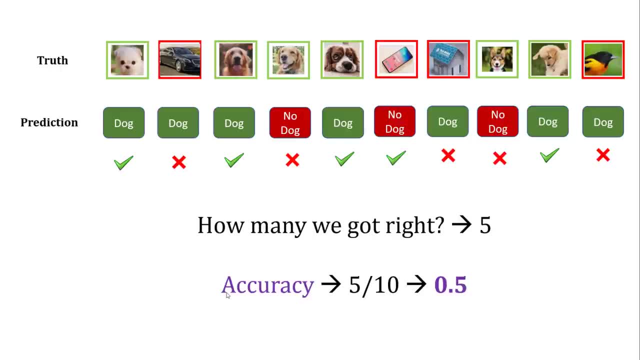 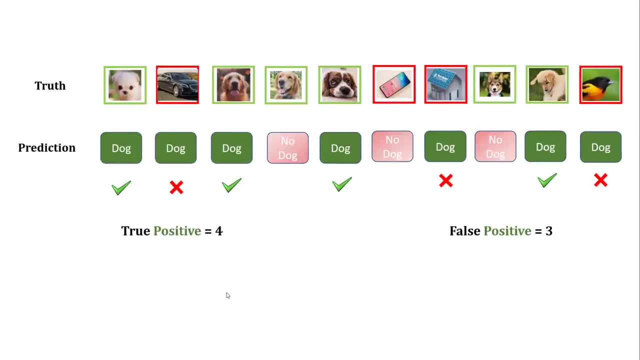 predictions. how many of your predictions you got it right. so we got five out of ten right hand and hence accuracy is 0.5. okay, now in this diagram again, we are going back to only positive class. so forget the no dog prediction. just take those out of your visualization. here we saw true, positive. 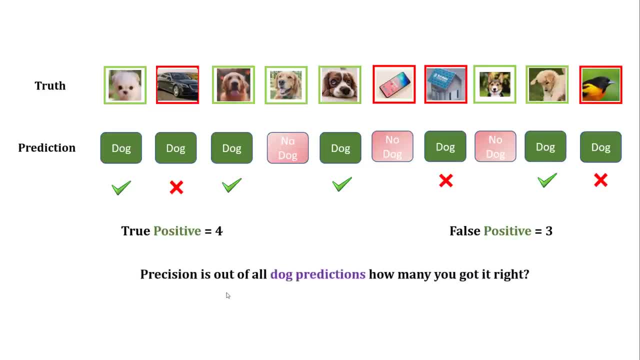 was four and false positive or three. so precision is out of all dog predictions, how many you got it right? so it is four by seven. so you have total seven dog predictions right. seven things. you predicted it to be dog. out of that, only four are dog. so that's why. 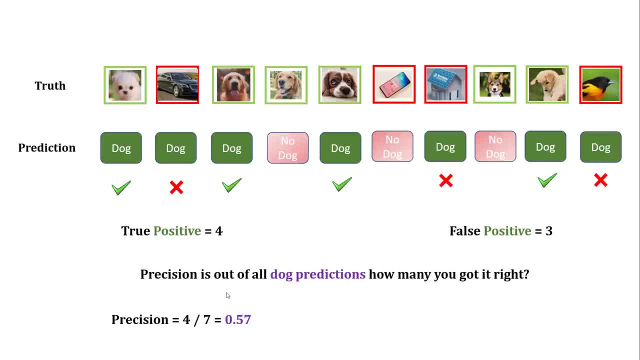 precision is four by seven point fifty seven. so this is the formula for precision: true positive divided by true positive, false plus false positive. okay, now let's talk about recall, so that when you are thinking about recall, you always think about truth as your baseline. so what is? 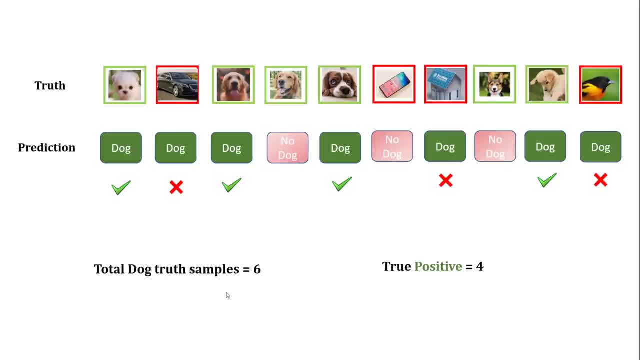 my truth, my, in my truth, total six samples are dog samples. okay, but when I predicted only I got four as correct predictions for dog. so recall is out of all your dog truth samples, how many you got right. so you had total six dog samples. out of that you got four right. hence four divided by six point sixty seven is. 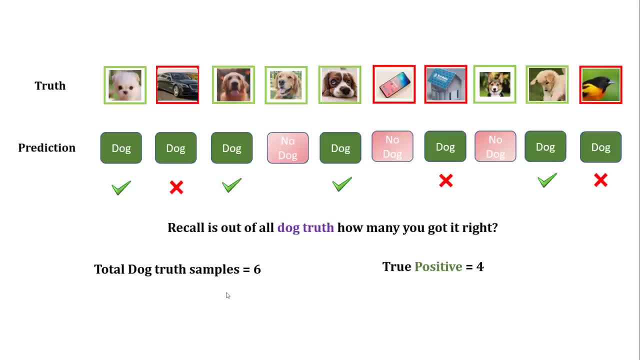 got right. so you had total six dog samples. out of that, you got four right. hence, 4 divided by 6.67 is your equal. okay, so recall is basically. here's my truth. okay, and in my truth, I have six dog samples. out of that, how many we are able to predict? 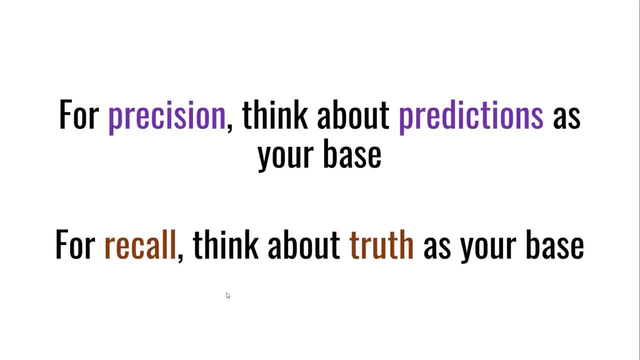 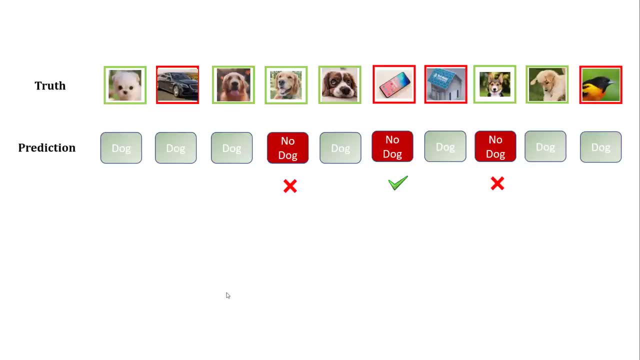 correctly. so now precision- recall has subtle difference, which is, when you're thinking about precision, always think about predictions as a baseline. when you're thinking about recall, think about truth as your base. now let's talk about the negative class. so, by the way, precision and recall is for individual. 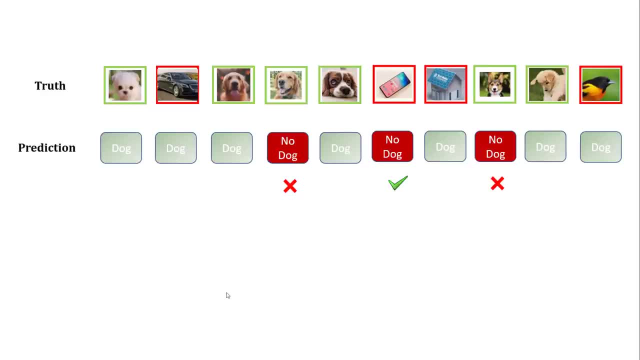 class. so the previously what we saw was precision and recall for dog class. now we are seeing precision and recall for not a dog class, so not a dog class. precision is 1 by 3 because when you're thinking about precision you are always thinking about predictions. so it's like: how many prediction do I have for no dog? 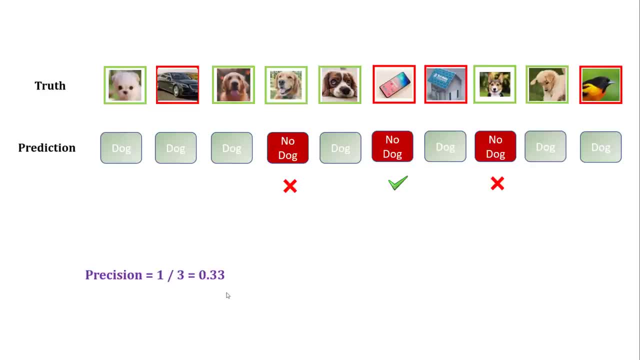 class? well, three, and how many of them are? are correct predictions? well, one, so 1 by 3. point 33: when you think about recall, okay, pause this video. try to guess what will be a recall for recall you think about truth is your baseline, okay, so, 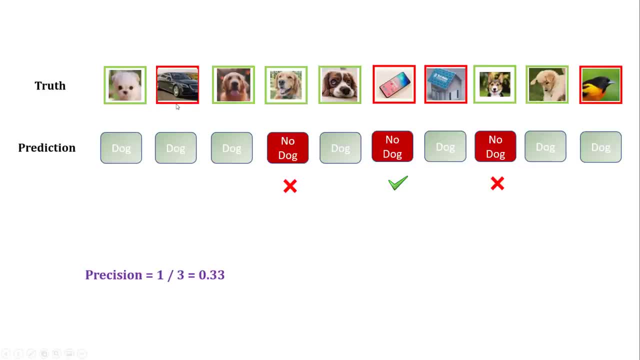 what is my truth? all right in my truth. how many no dog samples I have? well, one, two, three, four, and how many of them I got right? well, only one. see, there is a green check mark here. so out of four no dog images I had, I was able to predict only one image correctly, that's. 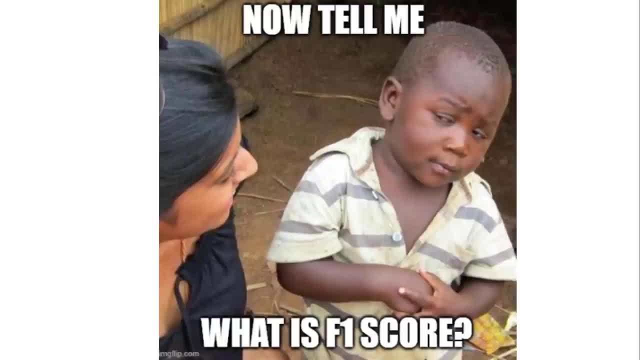 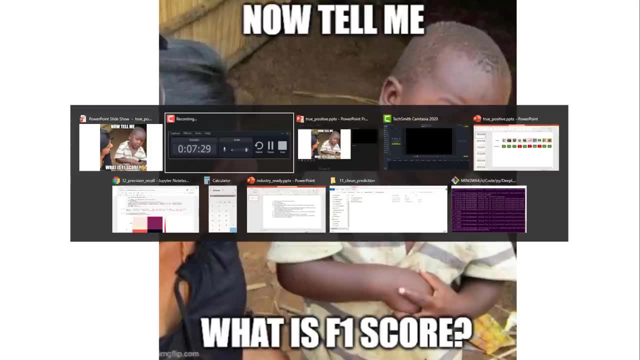 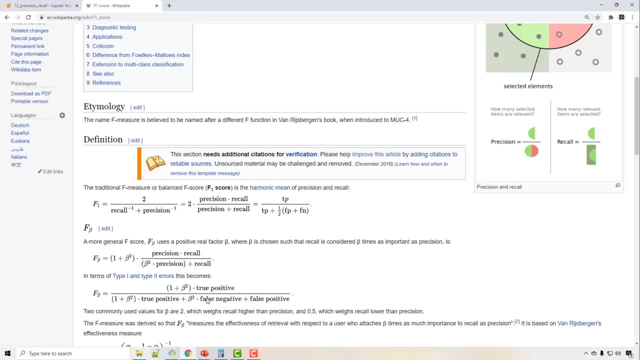 why 1 by 4 is 0.25. now you'll ask me what is f1 score? because you see f1 score everywhere, along with recall and precision, whatever, okay. so f1 scores definition on Wikipedia is 2 into precision, into recall, divided by 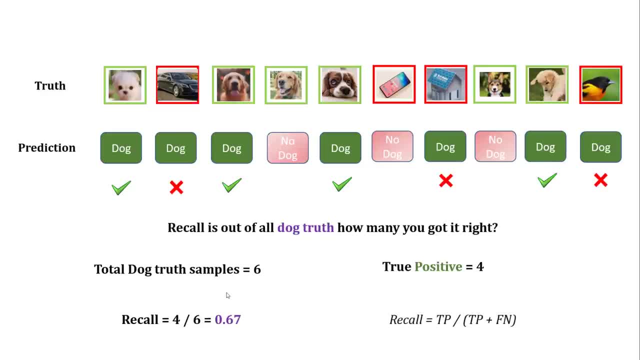 your recall okay. so recall is basically: you got four right. so recall is basically you got four right. so recall is basically: here's my truth, okay, and in my here's my truth, okay, and in my, here's my truth, okay, and in my truth I have six dog samples out of that. how. 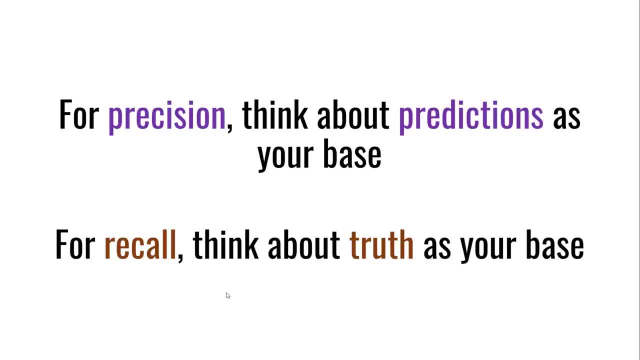 truth, I have six dog samples out of that. how truth- I have six dog samples out of that. how many we are able to predict correctly? many we are able to predict correctly. many we are able to predict correctly. so now, precision recall has subtle. so now, precision recall has subtle. 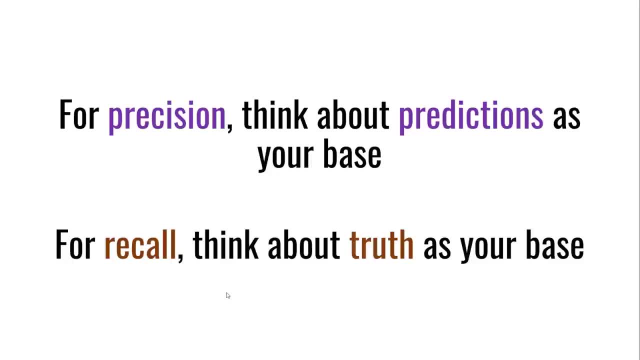 so now, precision recall has subtle difference, which is when you're thinking. difference, which is when you're thinking. difference, which is when you're thinking about precision. always think about about precision, always think about about precision, always think about predictions as a baseline when you're, predictions as a baseline when you're. 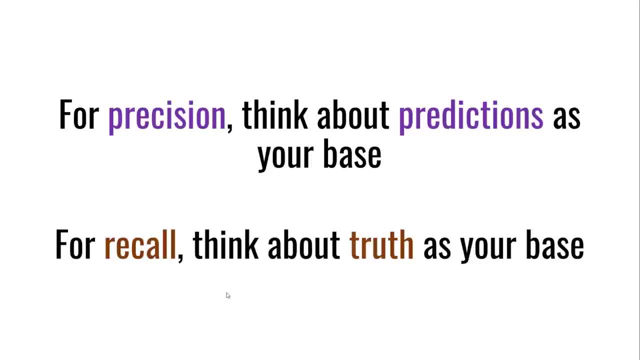 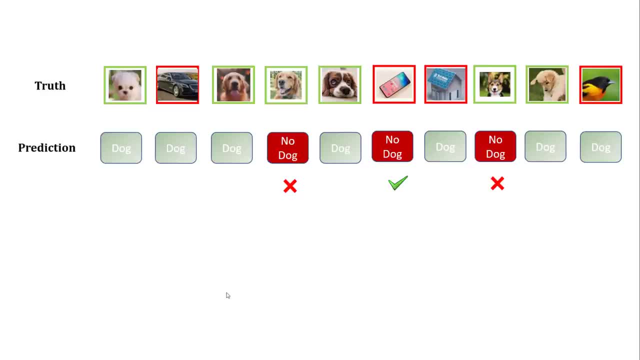 predictions as a baseline. when you're thinking about recall, think about truth as thinking about recall. think about truth as thinking about recall. think about truth as your base. now let's talk about the negative class. so, by the way, precision and recall is for individual class. so the previously what we saw was precision and recall for dog class. now we are. 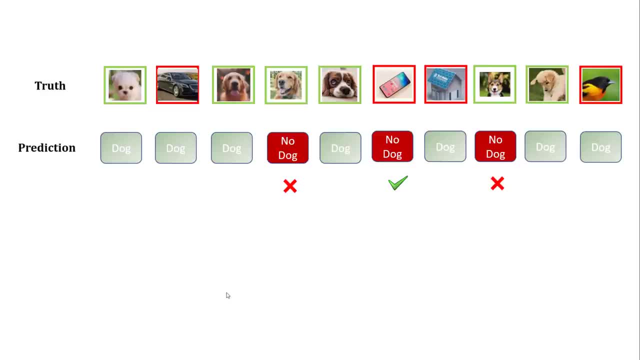 seeing precision and recall, for not a dog class, so not a dog class. precision is 1 by 3, because when you're thinking about precision you are always thinking about predictions. so it's like: how many prediction do I have for no dog class? well, 3, and how many of them are correct predictions? well, 1, so 1 by 3. point 33: 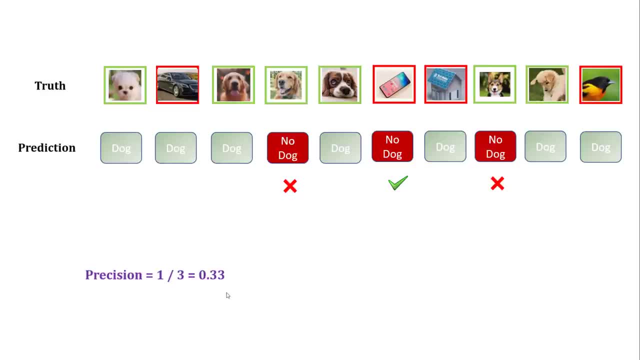 when you think about recall? okay, pause this video. try to guess what will be your recall. for recall you think about truth is your baseline. okay, so what is my truth? all right, in my truth. how many no dog samples I have? well, 1, 2, 3, 4 and how. 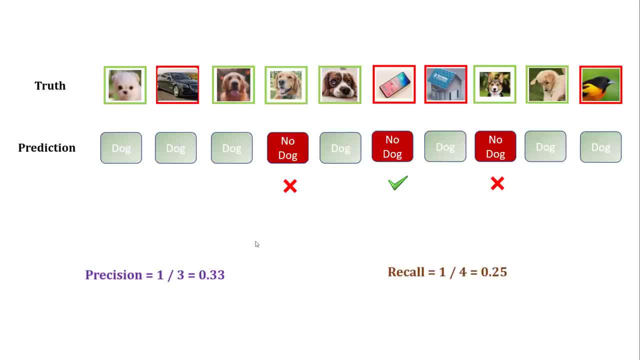 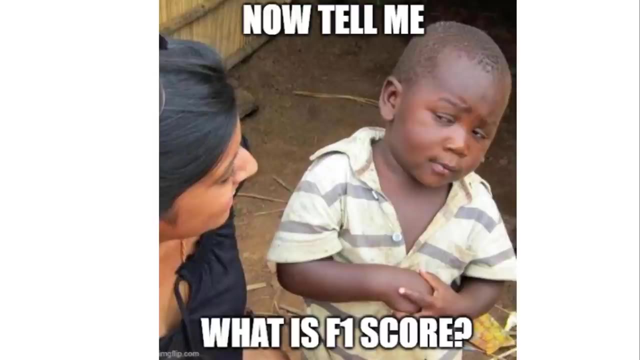 many of them. I got right right. well, only one. see, there is a green checkmark here. so out of four no dog images I had, I was able to predict only one image correctly. that's why 1 by 4 is 0.25. now you'll ask me what is f1 score? because you see f1 score. 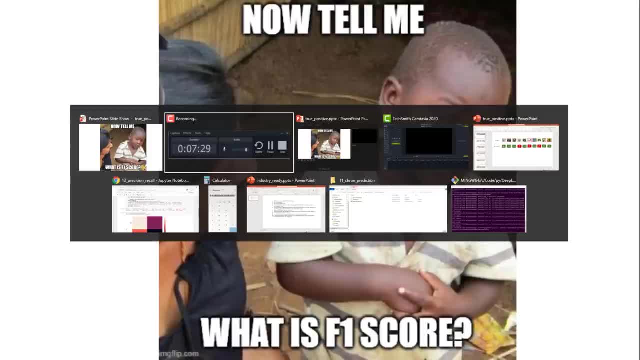 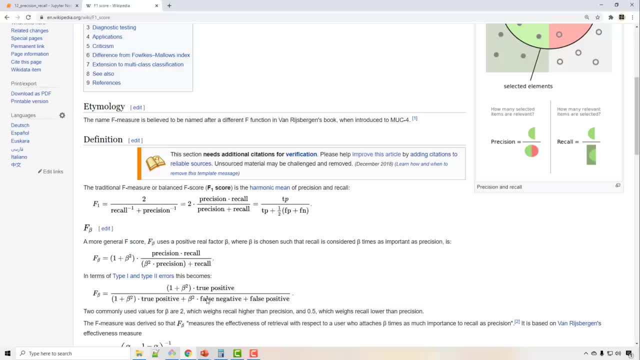 everywhere, along with recall and precision, whatever. okay so f1 scores. okay so f1 scores definition on Wikipedia is 2 into precision, into recall. divided by precision plus recall, it is just a harmonic mean of precision and recall it just gives you the overall health or overall performance of your model. so now 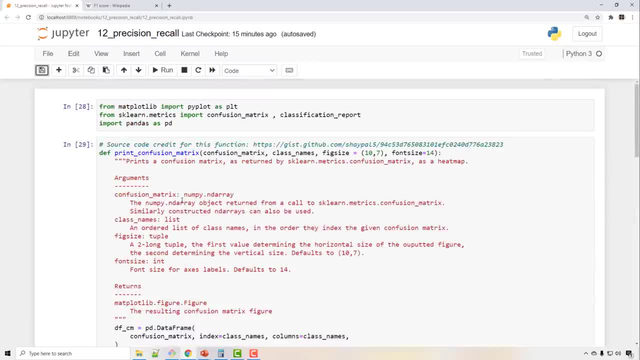 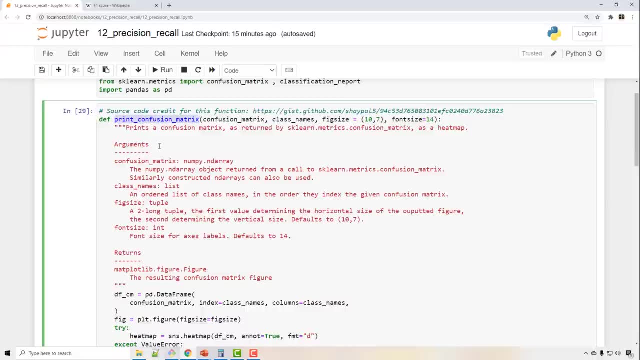 we are going to write some code in Python to check all these things, okay, so I imported some libraries in my Jupyter notebook and I have a written this function. actually, this function is a function that I have written in the work system of my��s, where it records special events like sometimes Iwanji. 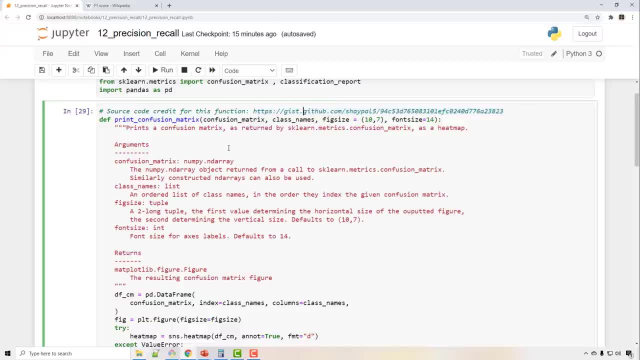 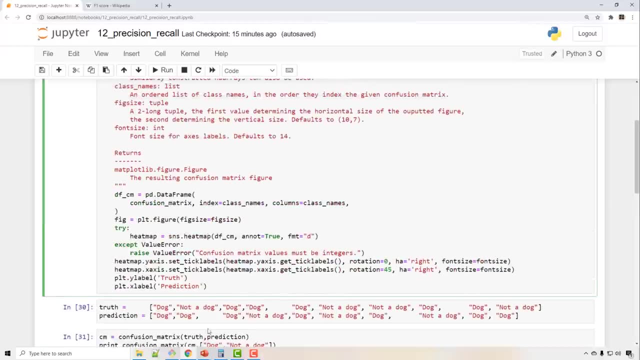 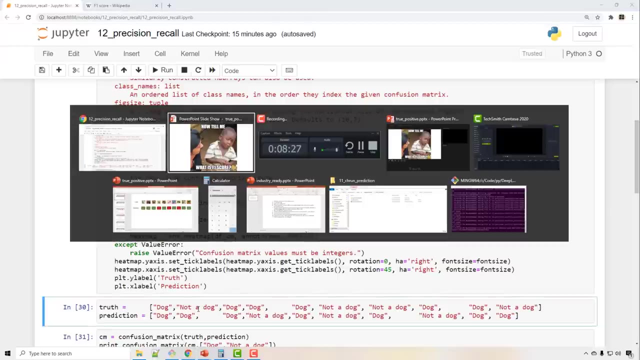 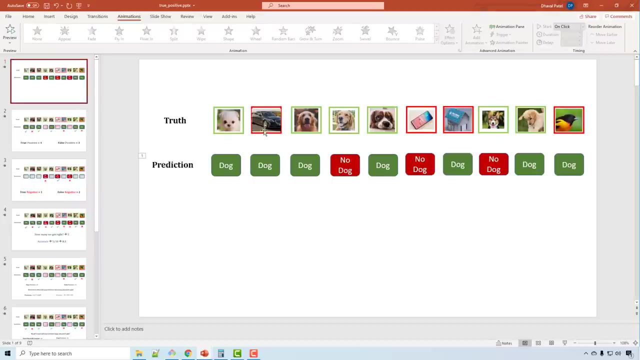 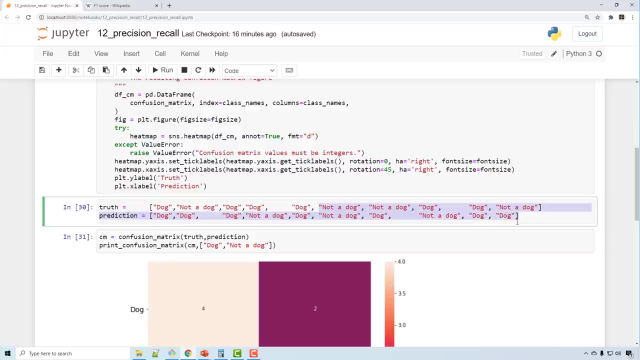 an right. so in our presentation that we had, see, we had dog no dog, dog, dog, dog. so see: dog no dog, dog, dog, dog, all right. and then prediction: okay, what was our prediction? dog, dog, dog, no dog. okay, dog, dog, dog, no dog. so that's what we have in truth and prediction. when you 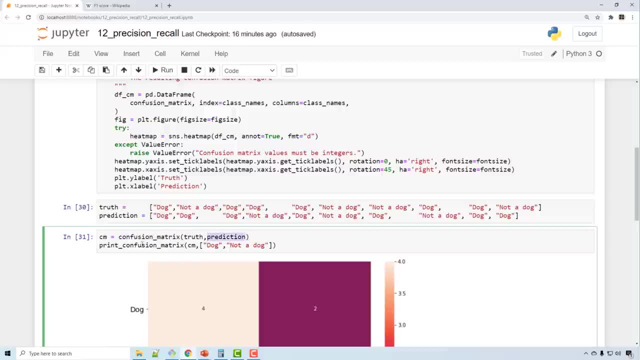 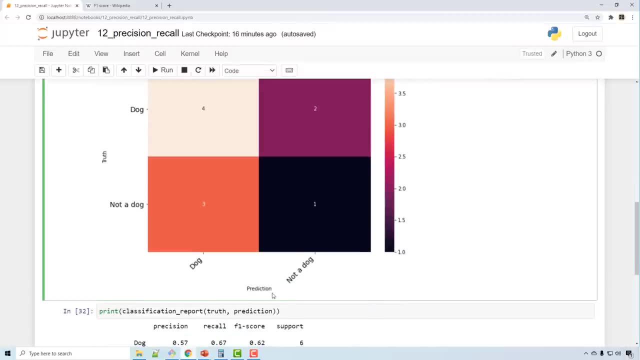 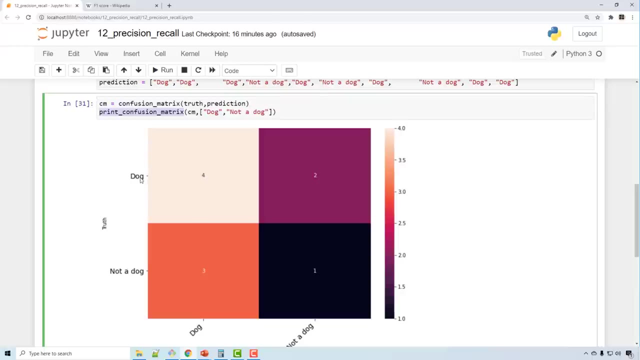 do confusion matrix, you need to supply truth and prediction, and when you print confusion matrix, this is how it looks like. so on the y-axis, you have truth, x-axis, you have prediction. what does this for means is: four times. I had dog as a truth and I predicted that to be a dog. so four times I. 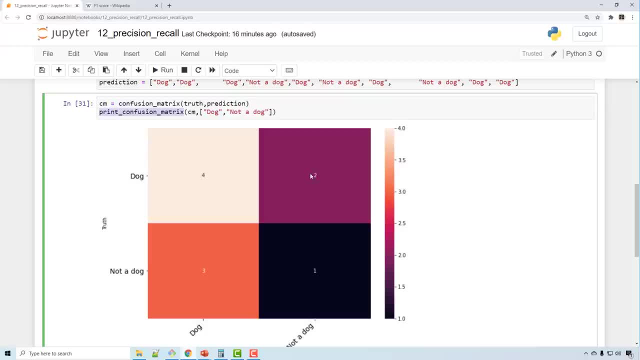 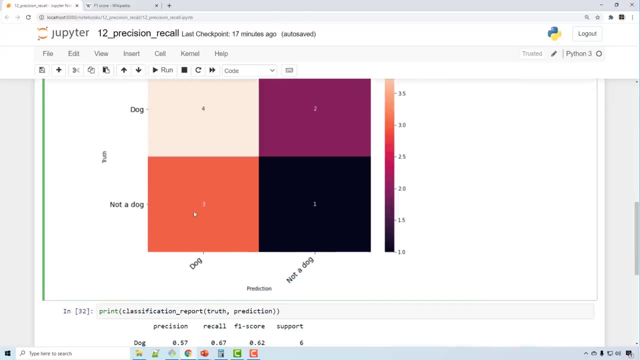 got it right. this is my true positive. two times the truth was dog. look at the y-axis. two times the truth was dog, but I actually predicted it to be not a dog, so I got it wrong. similarly, three times it was not a dog but I predicted it to be dog, and one time it was not a dog. I 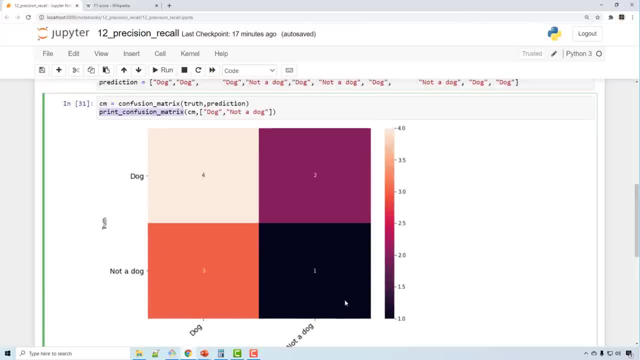 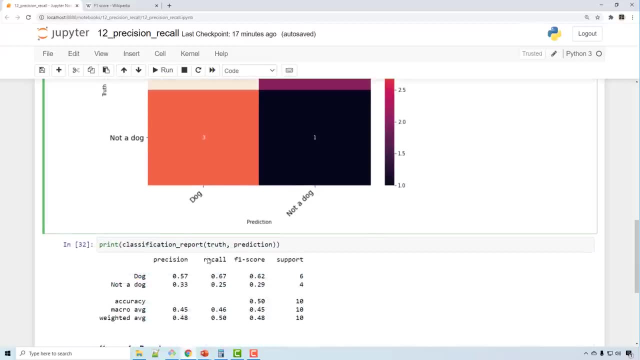 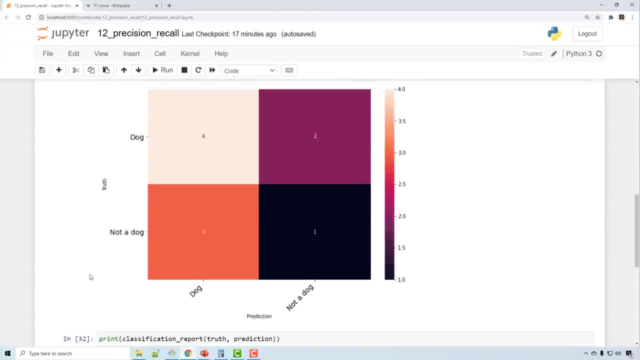 predicted to be not at all. so anything that you see on a diagonal, those are all correct predictions and these all are errors. so two and three is an error. okay, when you print a classification report using this function. so in in sk, learn, there is a classification report that you can. 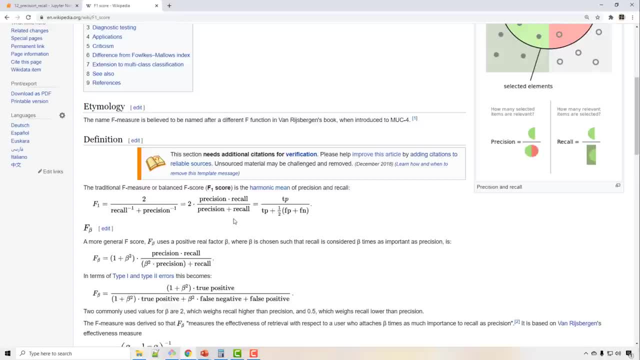 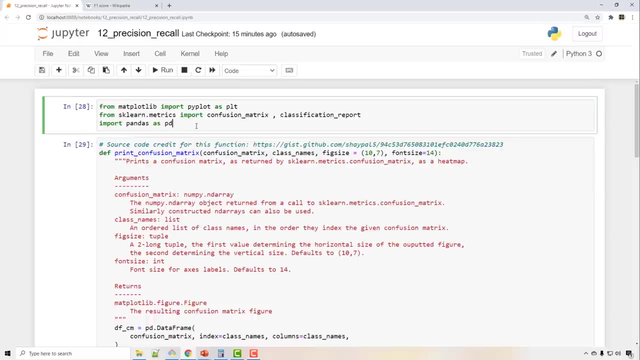 precision plus recall. it is just a harmonic mean of precision and recall it just gives you the overall health or overall performance of your model. so now we are going to write some code in Python to check all these things. okay, so I imported some libraries in my Jupyter notebook and I have a written this: 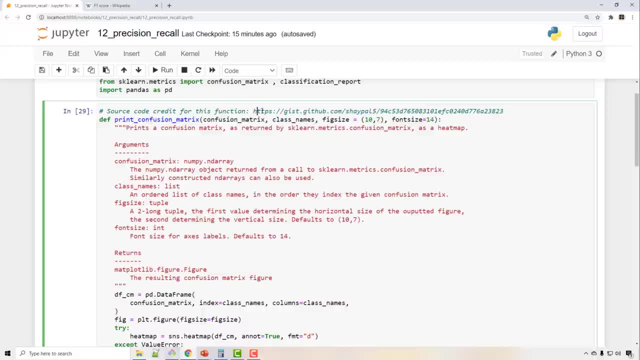 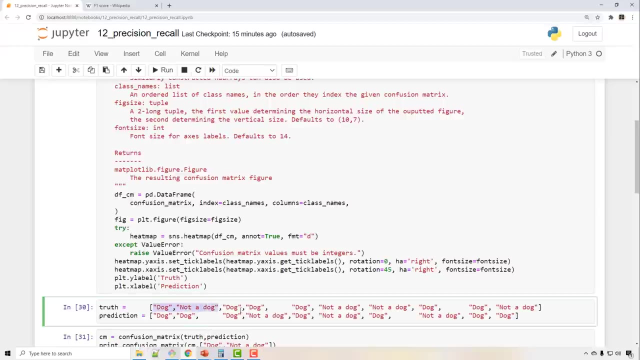 function, actually this function. I have sourced it from this gist, so thank you for whoever wrote this function, and it will just plot a confusion matrix. confusion matrix is. let me show you what is confusion matrix. okay, so I have all this sample so we can. dog not a dog. these, these are the same. 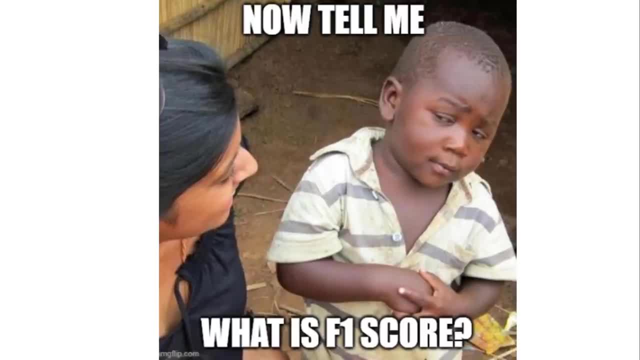 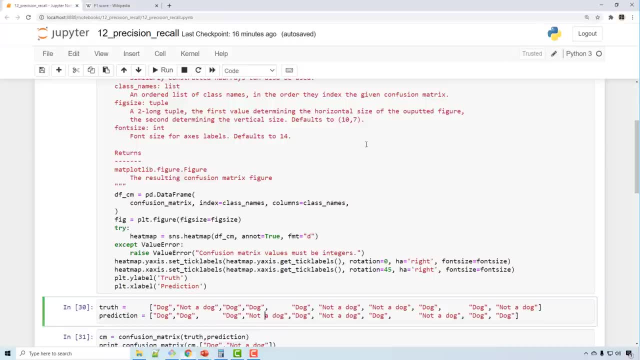 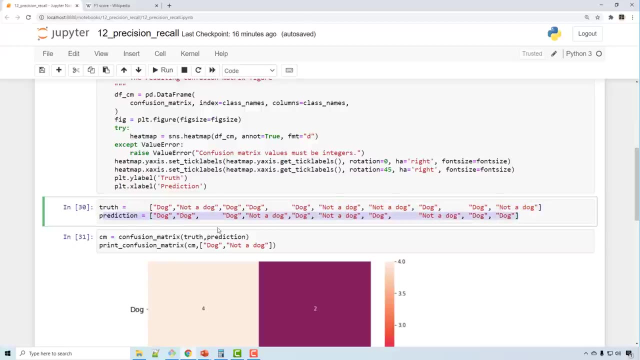 samples that we saw in our presentation. right so, in our presentation that we had, see, we had dog, no dog, dog, dog, dog. so see, dog, no dog, dog, dog, dog, all right. and then prediction: okay, what was our prediction? dog, dog, dog, no dog. okay, dog, dog, dog, no dog. so that's what we have in truth and prediction when you do. 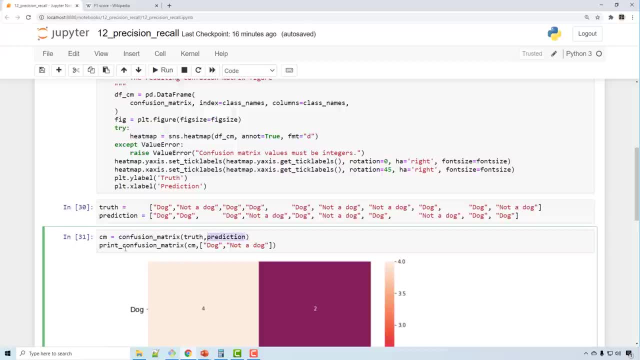 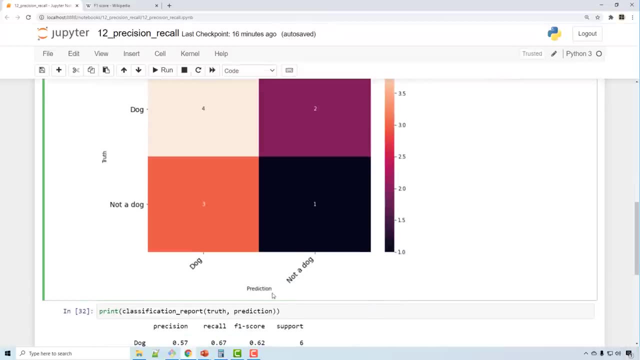 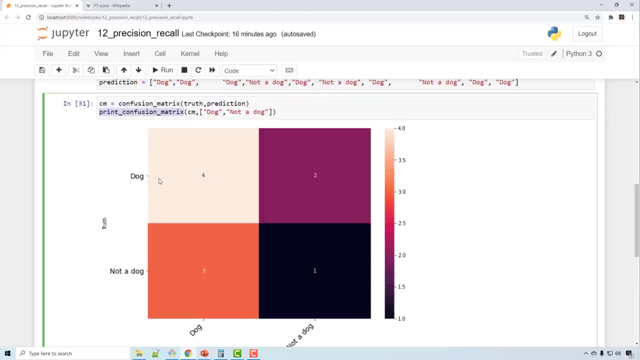 confusion matrix, you need to supply truth and prediction, and when you print confusion matrix, this is how it looks like. so on the y-axis you have truth. x-axis, you have prediction. what this for means is four times I had dog as a truth and I predicted that to be a dog. so four times I got it right. this is my true positive 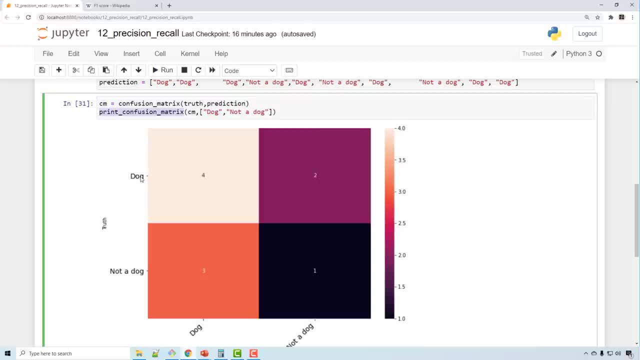 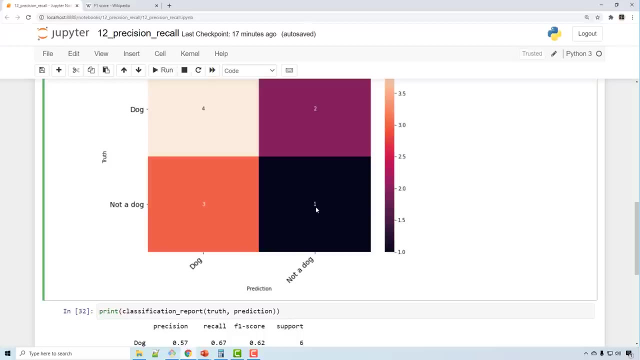 two times the truth was dog. look at the y-axis. two times the truth was dog, but I actually predicted it to be not a dog, so I got it wrong. similarly, three times it was not a dog, but I predicted it to be dog, and one time it was not a dog. I 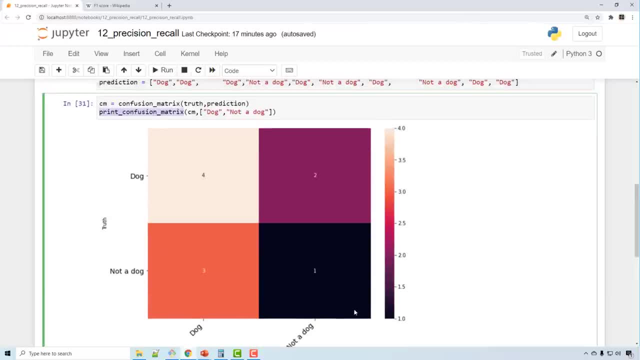 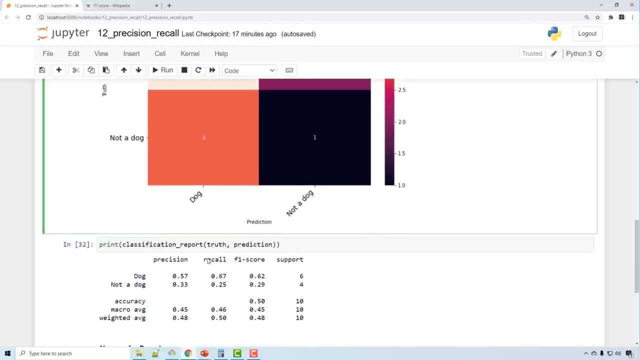 predicted to be not a dog. so anything that you see on a diagonal, those are all correct predictions and these all are error. so two and three is an error. okay, when you print a classification report using this function, so in in a scale on, there is a classification report that you can after building your machine.